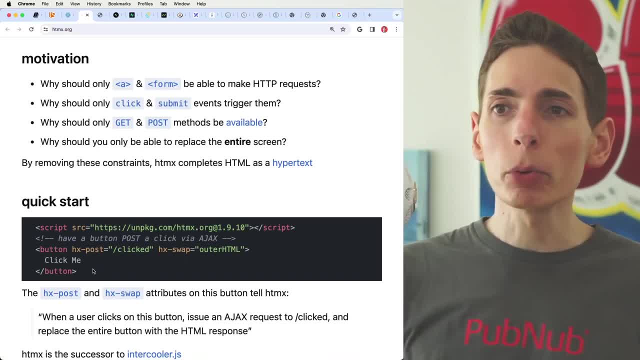 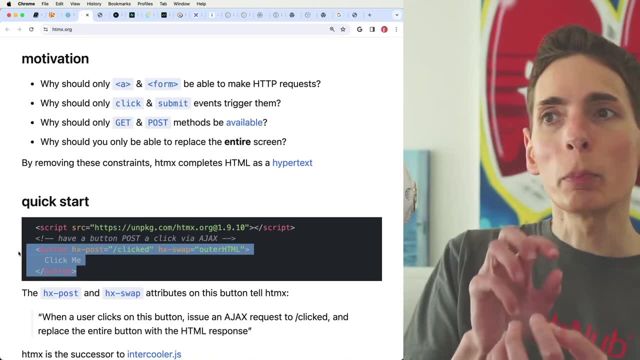 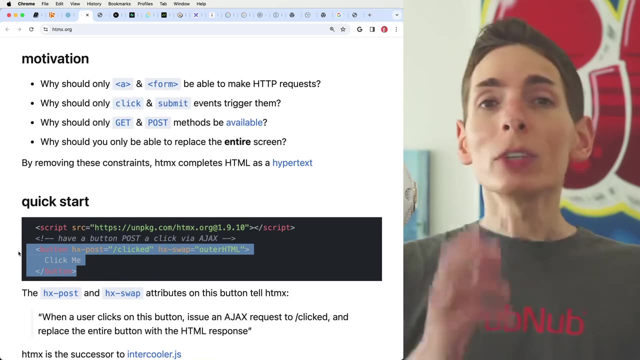 software engineering. really, You just have to write some simple markup and then it will. the framework in the backend will take care of everything for you. Now this is. it does require you to build your code and your server. in a certain way, Though your front-end now becomes accessible to more, because you don't. 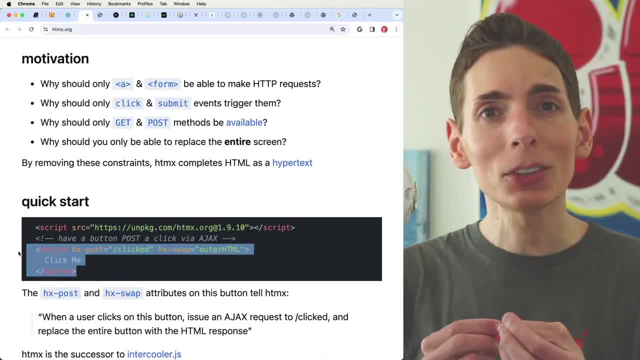 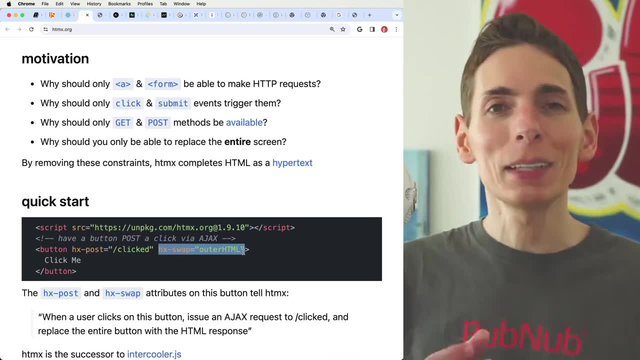 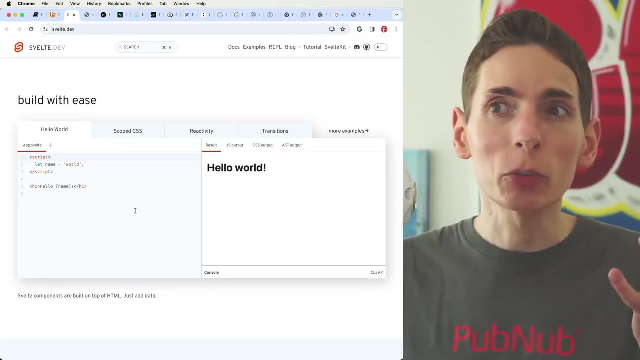 need to know JavaScript, You don't really need to know coding practices. You can just use HTML and simple markup attributes, Tags in order to describe how the page is going to be interacting with a server API. Then, of course, at number three, we have Svelte. Now Svelte is going to be more in competition with React, because it is a sort of a 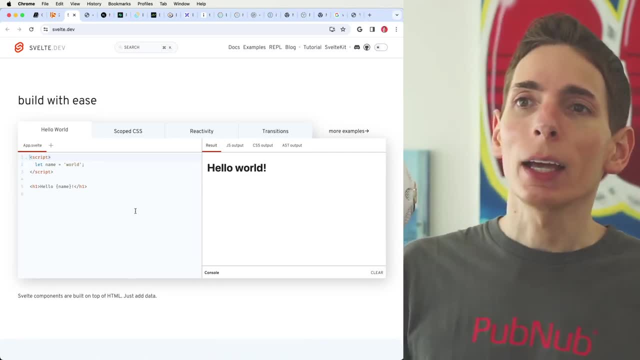 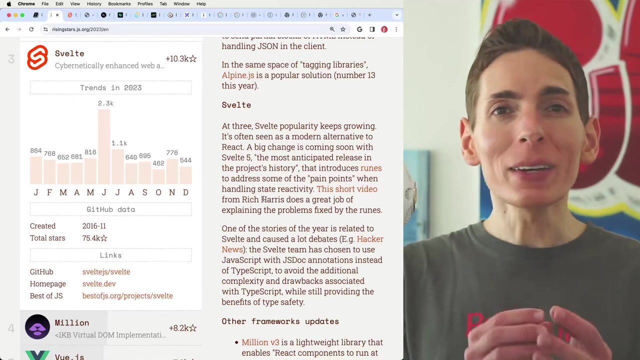 component driven, fully orchestrated front-end framework And it's going to give you the same with templates and your ability to write code. It is cleaner. I do like there's less indentation here, And so you've got this. like you know, contained Svelte file. You can also have a contained CSS, which is great. And number three, the most, 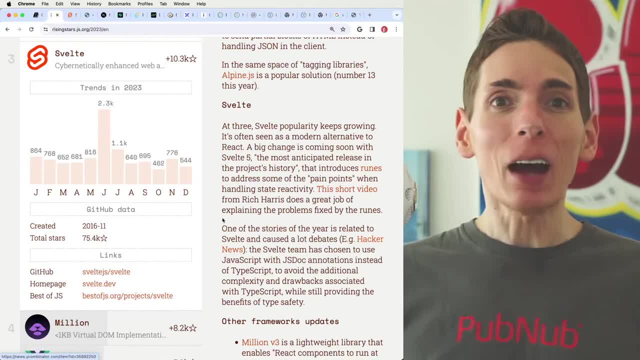 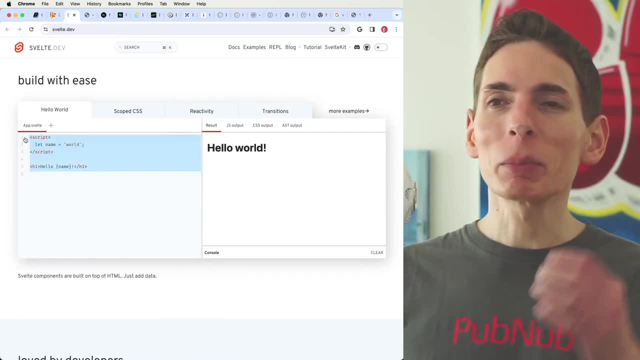 popular front-end JavaScript frameworks. we have Svelte, which is going to be competing directly with React. What I like about Svelte is it's a lot cleaner from a syntax perspective, right It's. I like it because there's less indentation and it. 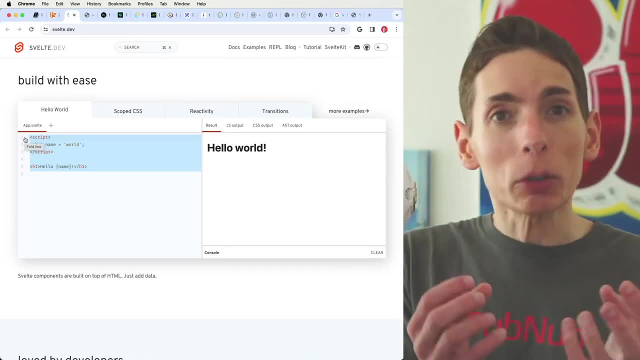 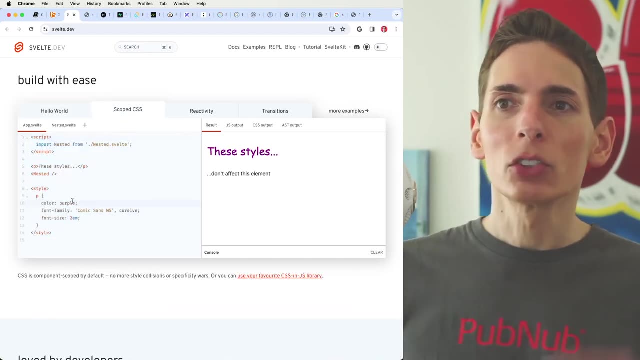 keeps the code clean, And what's great also is that it's just like React. everything's self-contained and sort of like. it's nice Svelte file, like a single file, And you do need to often have styles and data layer presentations in the 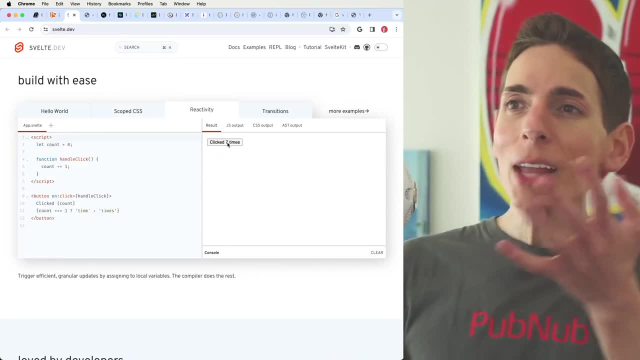 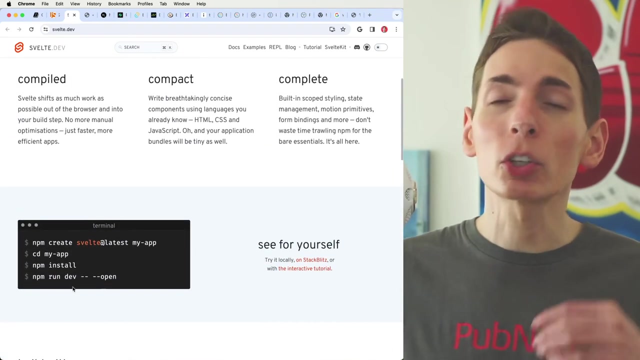 code And it's great to sort of merge all that together, even state, So it helps you keep state a little more simply. Oh, this is great. It's clean, You can kind of see where things align with each other, less indentation And as a bonus it's going to be faster overall. It's just built from because React, I mean, if you've 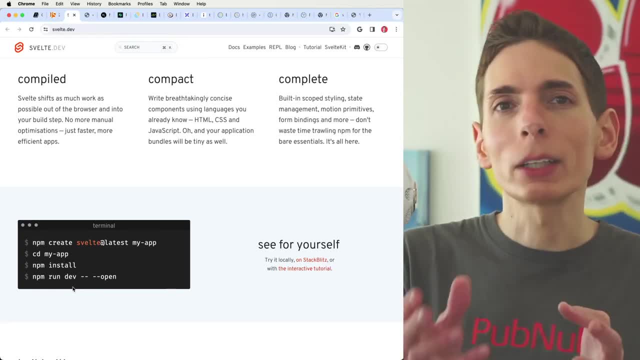 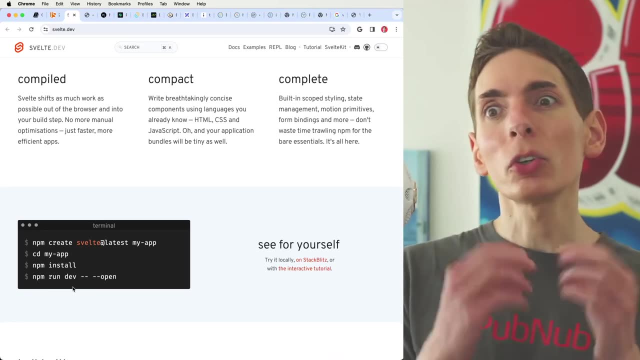 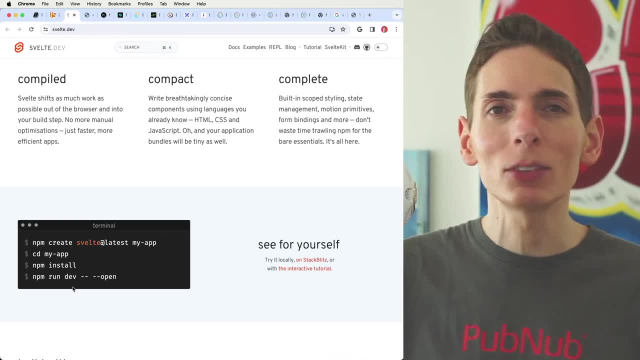 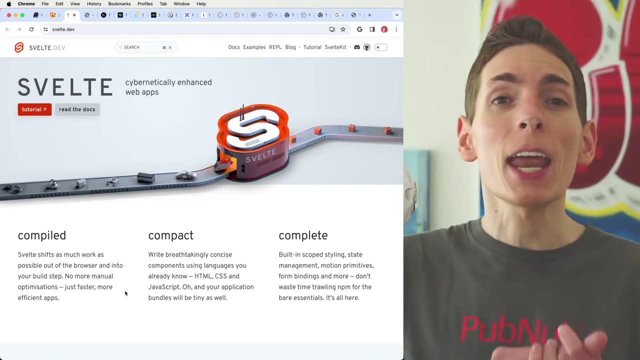 So it's going to be a little bit slower. So it's going to be a little bit slower, So it's not going to be as fast. It's just vanilla JavaScript and CSS. that is, I would say, the next step up. So if you're thinking of a nice alternative to React, Svelte is probably going to be an. 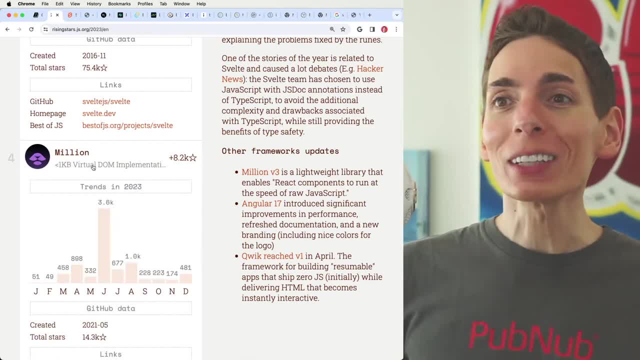 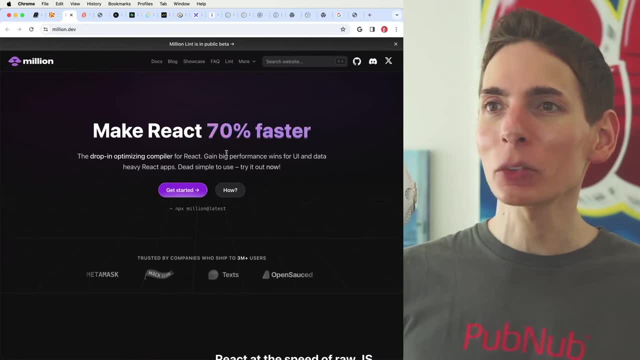 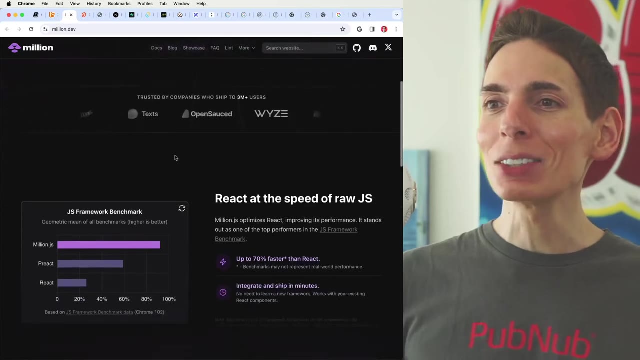 excellent choice. Then we have million less than a kilobyte virtual DOM implementation. No way Make React 70% faster. Drop-in optimizing compiler for React. Oh, I was just talking about how React was so slow. Well, if you use million, apparently you can just. 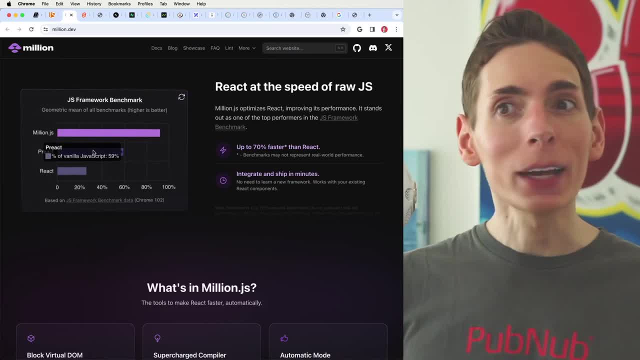 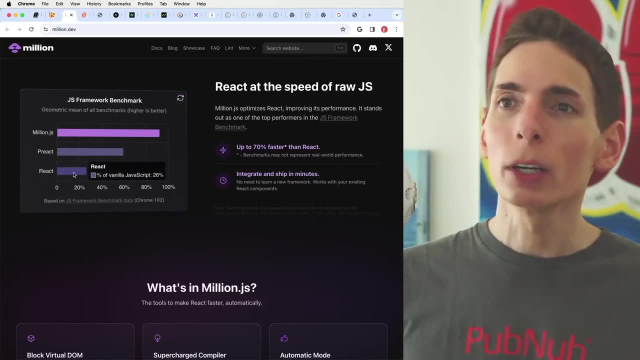 Bypass all that, All right. so preact is sort of a rewrite. so if we look at this list here we've got benchmarking with javascript react itself pretty darn slow. i've it's a. it is slow. then you've got preact, which 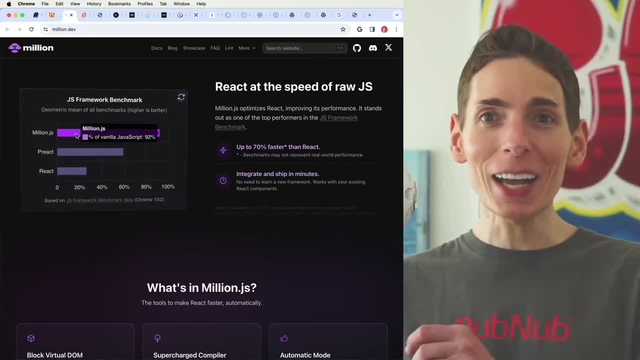 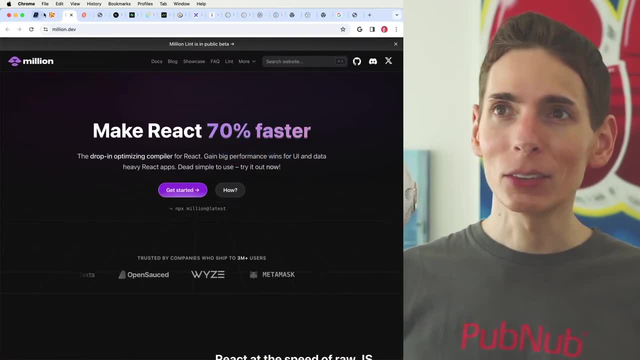 looks like it's twice as fast, but if you pipe in million js it's gonna go even faster. all right, well, if you're looking for that speed, let's drop in some optimization here. you can see why that is. that's definitely gonna be popular there. and then then you've got view js, which is a another. 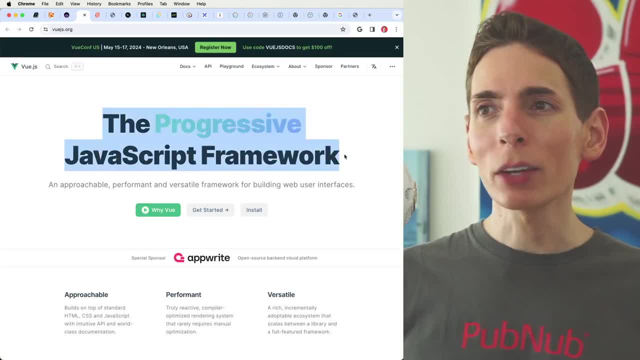 competitor to svelte and react. it says it's progressive, which means, you know, tries to only load what's needed from the user's in perspective, which is great because that's going to be a faster user's experience. the browser has to download less. it has to come render less. it has to interpret. 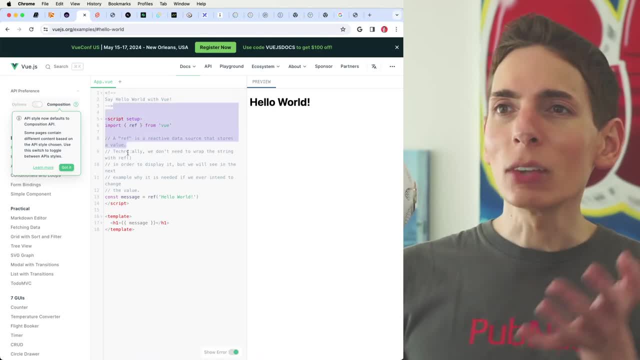 less, which means it's a faster user experience. the the examples they have here are similar to svelte, for example, where they it's nice separation concern, but it's all a nice one file, excellent pattern, really good pattern. i love it. yeah, this is fantastic. so this is. 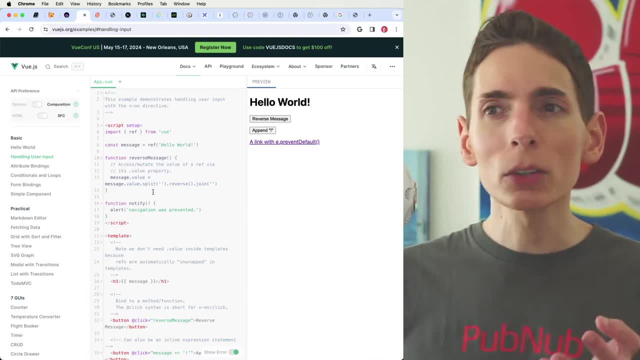 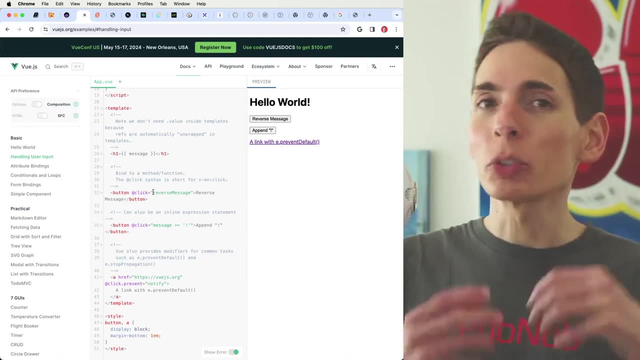 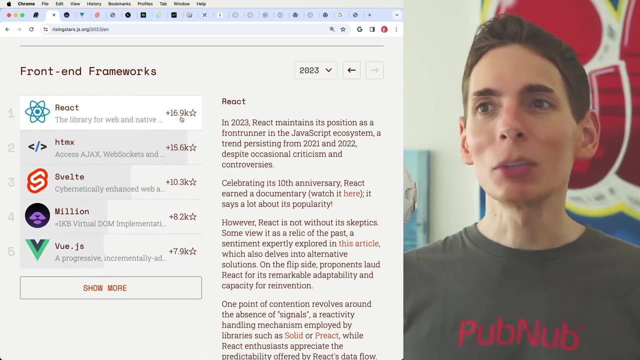 uh, view is very similar to svelte from that perspective- nice and clean. so svelte and view would definitely be closer competitors compared to react, although all three of them are options when you're building application experiences for end users. front-end frameworks are going to be react, hdmx, svelte, million and vue js. so we see we've got two, two react related items here: million. 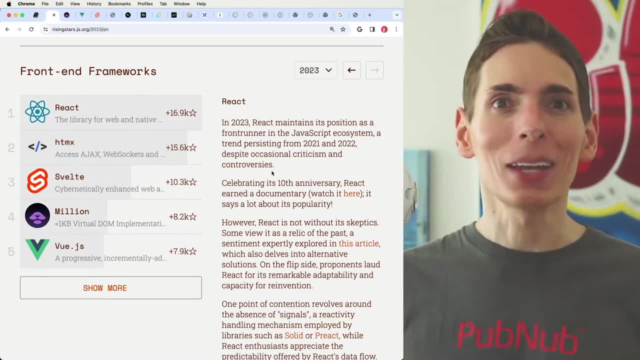 and react. so just add in million to react and you'll get a better react. 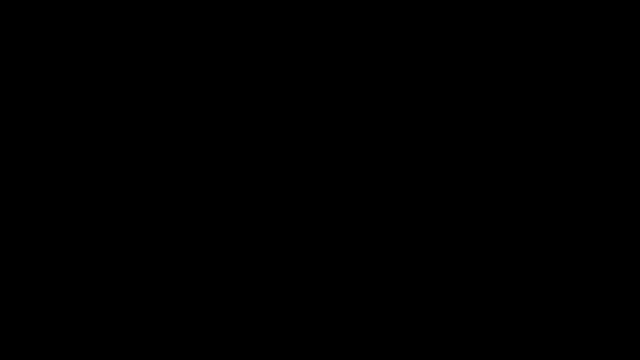 Let's see if we can prove to ourselves some more reasonably interesting transpose properties. So let's define some matrix C that's equal to the sum of two other matrices, A and B, And so any entry in C I can denote with a lowercase cij.